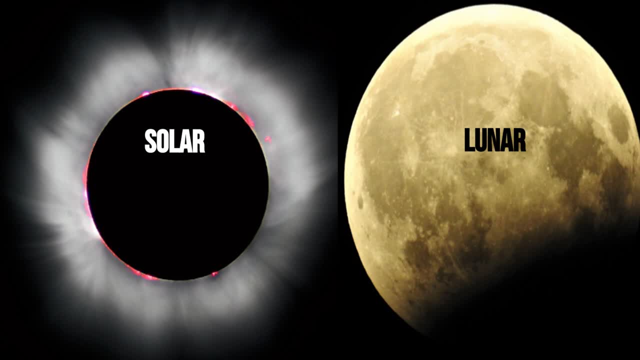 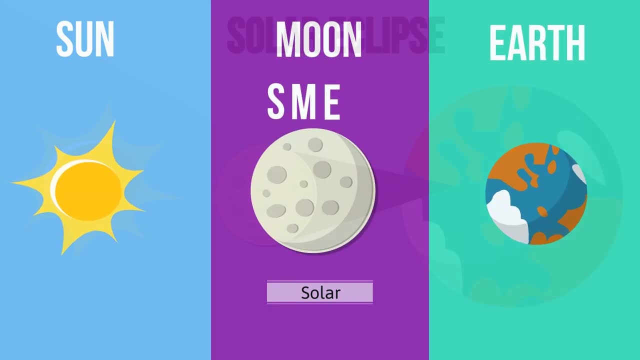 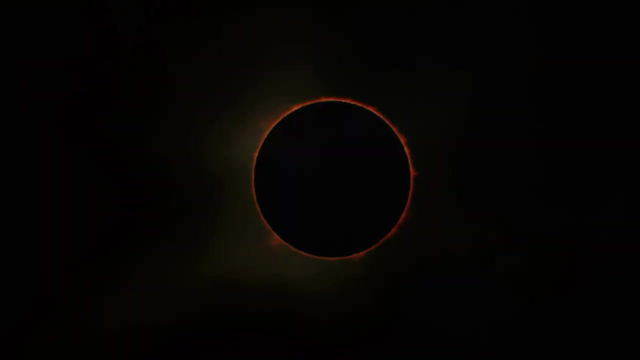 lunar eclipse. The order of the celestial bodies during a solar eclipse is the sun, moon and earth, or SME. Also, please remember that the shadow of the moon only falls on a small portion of the earth and people in this portion can look towards the sun to see the solar eclipse. 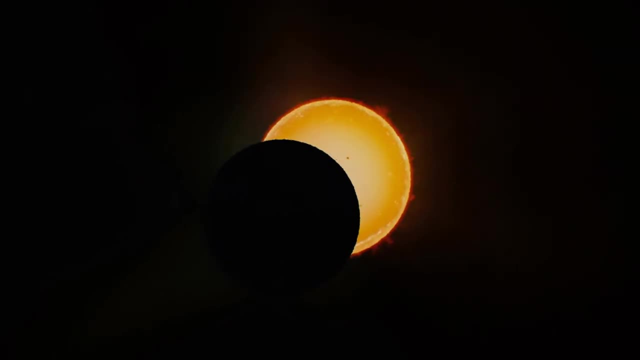 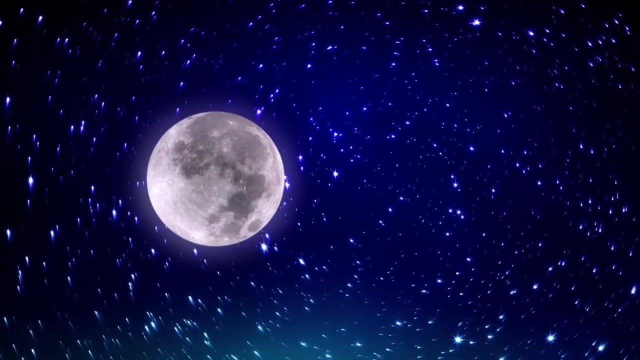 Remember: never look directly at the sun. That's not healthy. Here's the path of the 2017 solar eclipse. Here's the path of the 2017 solar eclipse. Here's the path of the 2017 solar eclipse. Notice how narrow the path is. During a lunar eclipse, the order of the celestial bodies is: 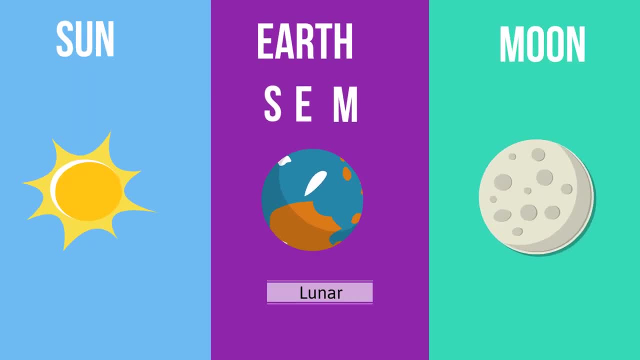 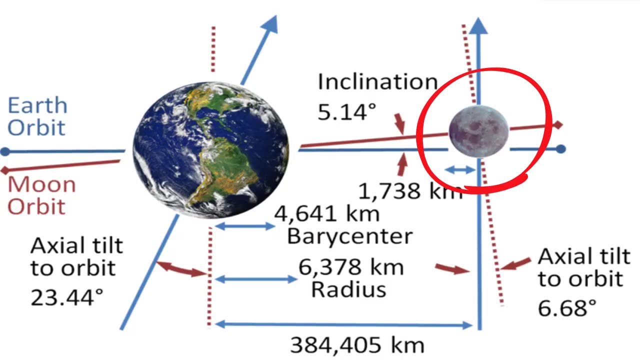 sun, earth, moon or SME. Next, you may be wondering why don't we see a solar and lunar eclipse every month. The reason is the moon's orbit around the earth is tilted about 5 degrees relative to the orbit of the earth around the sun. This tilt is just enough to 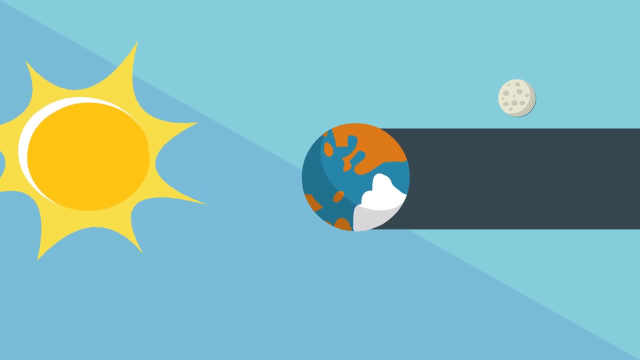 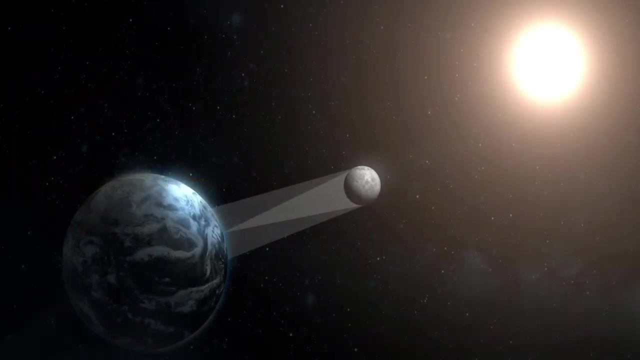 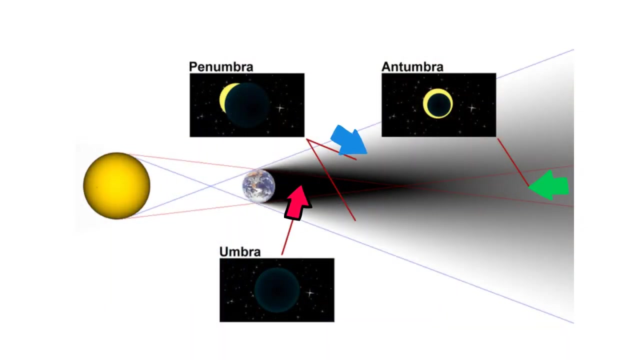 place the moon out of the earth's shadow for most full moons and the earth out of the moon's shadow for most new moons. When the earth, moon or earth is blocking the sun, three types of shadows are created: The umbra, penumbra and the antumbra. The umbra is the shadow's dark core. 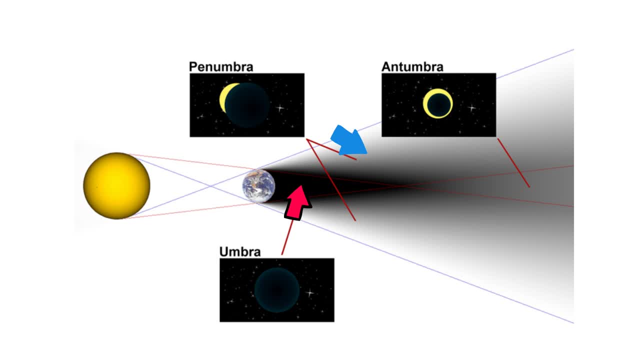 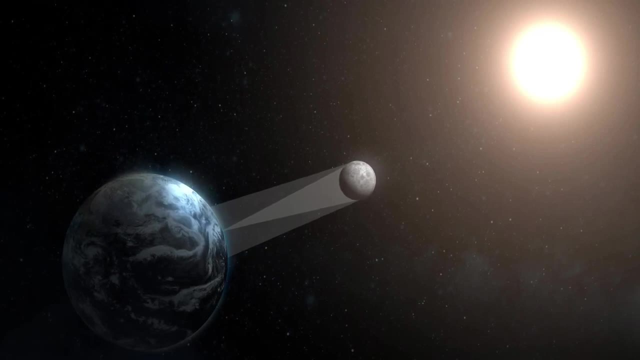 The penumbra is the less dark outer part of the shadow surrounding the dark core, And the antumbra is the lighter area of the shadow that appears beyond the umbra. These different types of shadows can cause different types of solar eclipses. There are three main types of solar 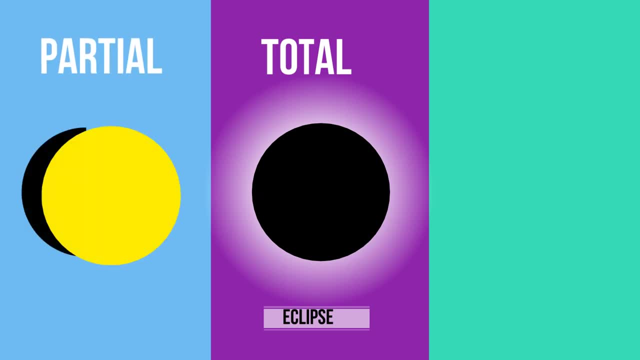 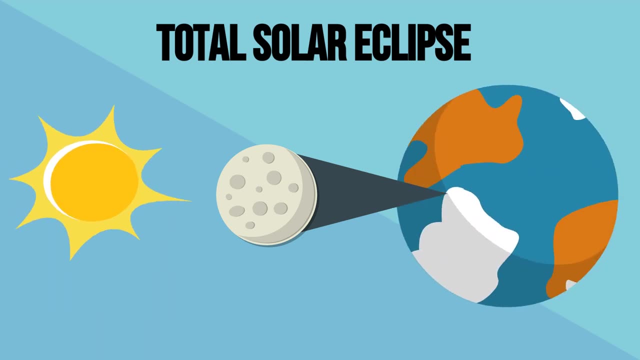 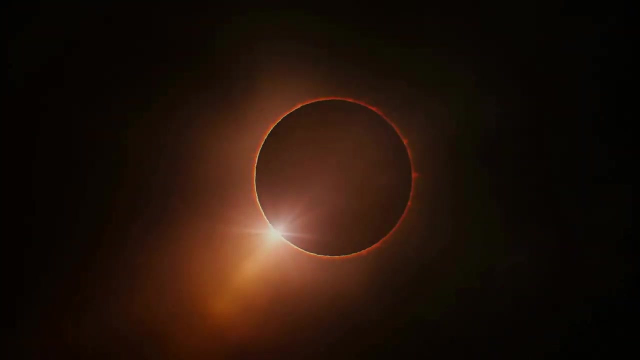 eclipses: The total, partial and annular. A total solar eclipse occurs when a small portion of the earth that the umbra covers, The sun, is covered for a brief period of time and it will become dark. A partial solar eclipse occurs when the umbra does not hit the earth or in the region of the 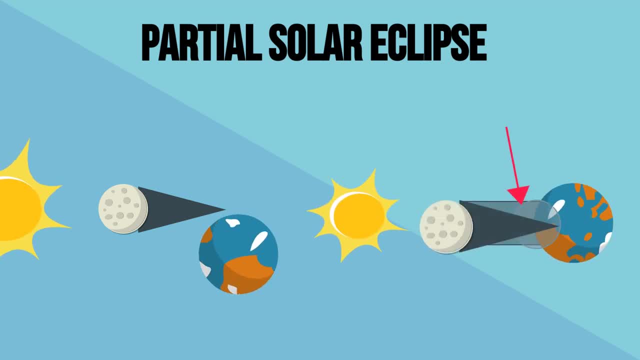 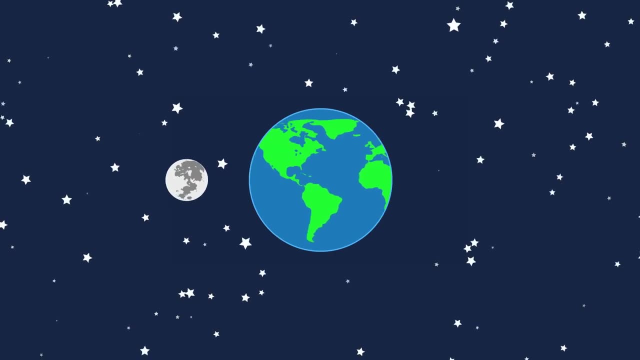 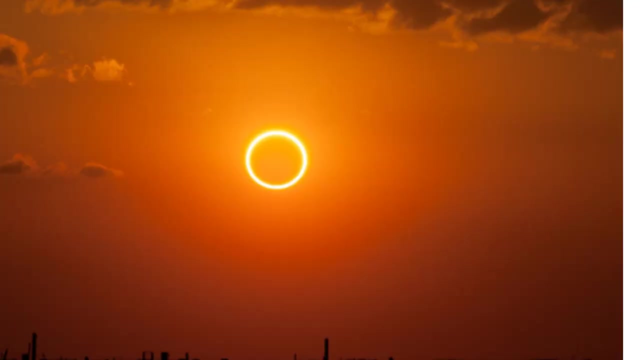 penumbra during a total eclipse. An annular eclipse occurs when the moon is near the furthest point from the earth, called the apogee, and the moon does not block out the sun completely. And here's what it looks like. There are also different types of lunar eclipses. 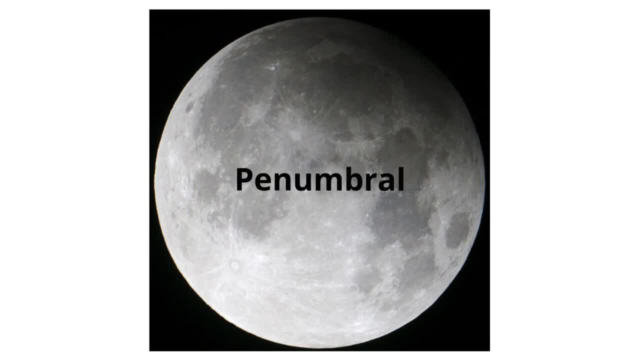 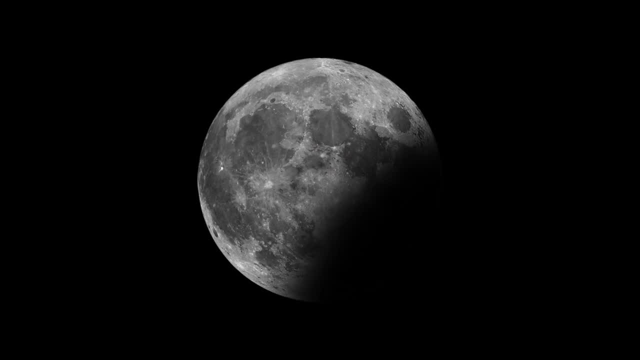 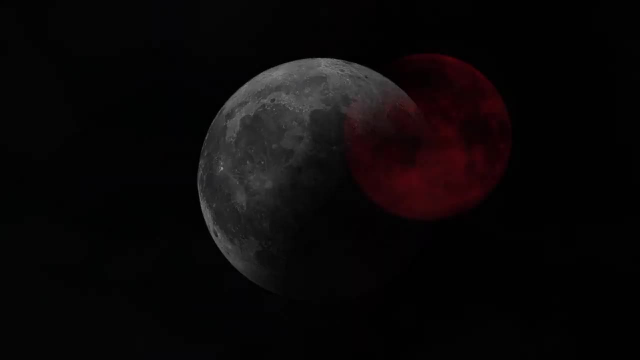 A penumbral lunar eclipse is when the moon passes through the earth's penumbral shadow. A partial lunar eclipse is when a portion of the moon passes through the earth's umbral shadow, And here's what this looks like. And then, finally, you have a total lunar eclipse where the entire moon 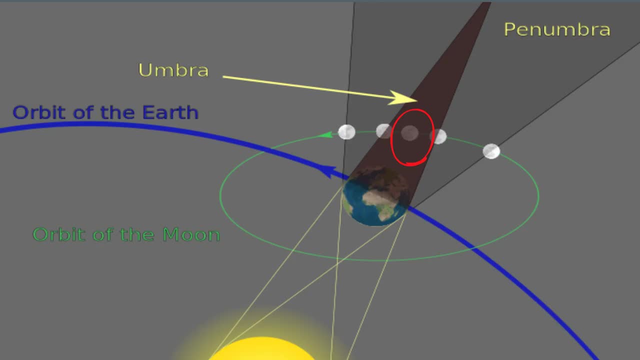 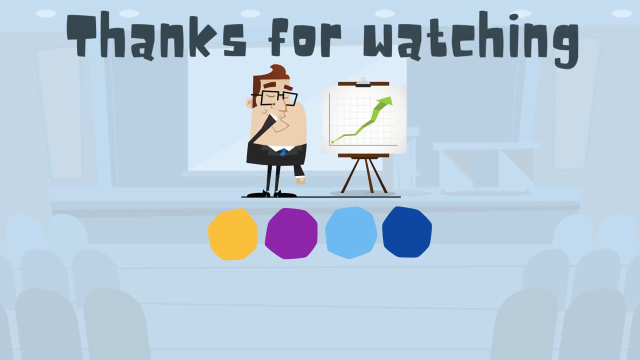 passes through the earth's umbral shadow. If you'd like to know more about eclipses, this playlist will help And, as always, thanks for watching. and MooMooMath uploads a new math and science video every day. Please subscribe and share. 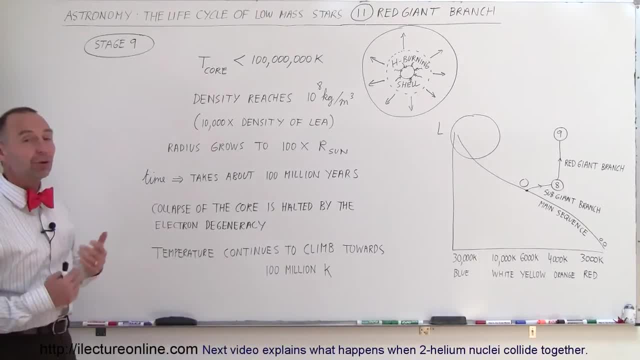 Welcome to Electron Line. and now we're getting to the next stage in the evolution of a star. It was the main sequence for billions and billions of years. Finally, the hydrogen fusion into helium stopped in the core. The core began to collapse. That additional heat began to fuse. We gave enough. 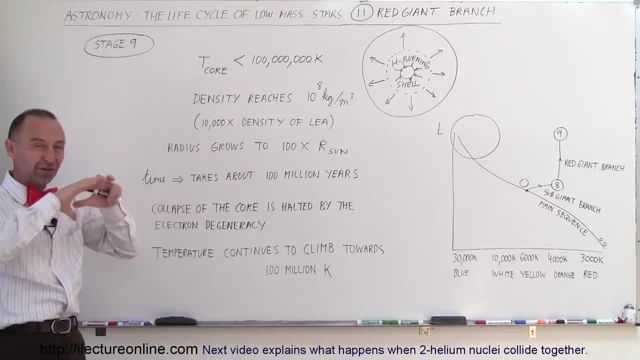 heat to the layers around the core. for that, for those layers, It's called the shell around the core. for that shell to begin to burn hydrogen into helium or to convert hydrogen into helium, That additional heat began to expand the star into larger and larger star Temperatures in the 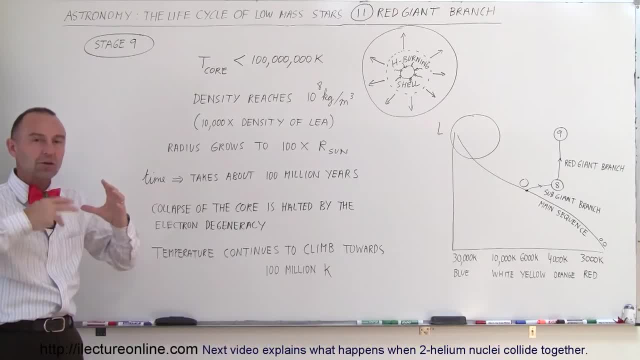 core continued to go up because the collapse of the core continued to drive that gravitational potential energy into heat, and so that was a sub-giant stage. and then what happened was, eventually the core collapse was halted. Something stopped the relentless pushing of the gravitational force, pushing the core ever into a smaller, smaller volume. but at some point something happened. 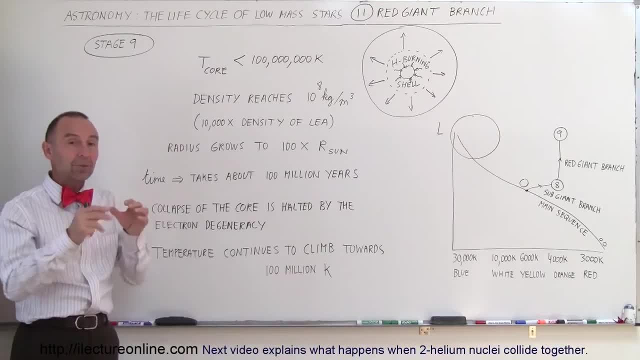 The electrons within that core because it's filled with helium, but there's for every helium nucleus there is. there are two electrons, and all those free-floating electrons between the helium nuclei began to repel each other more and more, more and more strongly, because, as they get closer and closer, 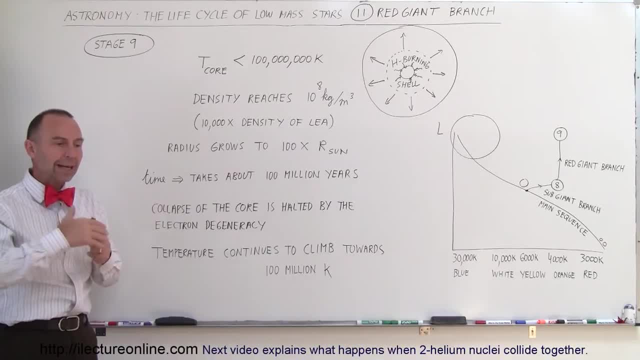 together, the repulsive force between the electrons began to grow. Electrons, they exist as waves. they create their own little volume sphere within the, the particular region within the core, and when those spheres begin to interfere with each other, they start to repel each other more and more.